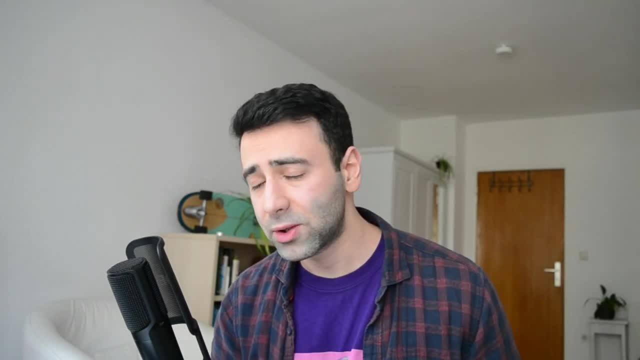 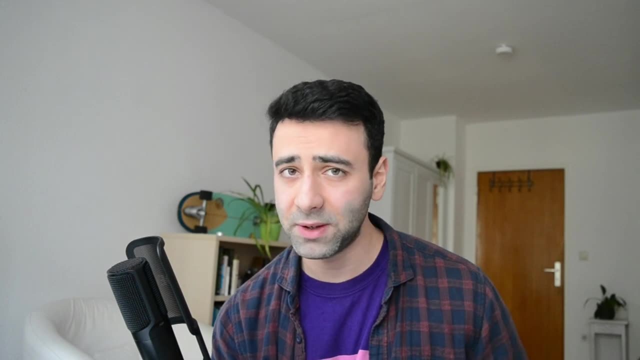 because it's very similar to object-oriented programming. So, for example, you want to fetch the user data, You can have users in your URL And if you want to fetch the specific data of a specific user, you put user slash ID and you fetch the data for this. So what are the good? 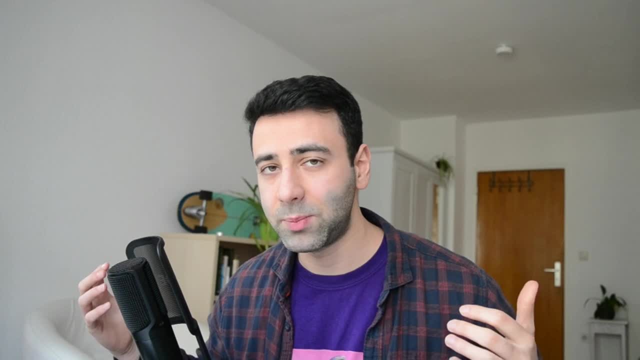 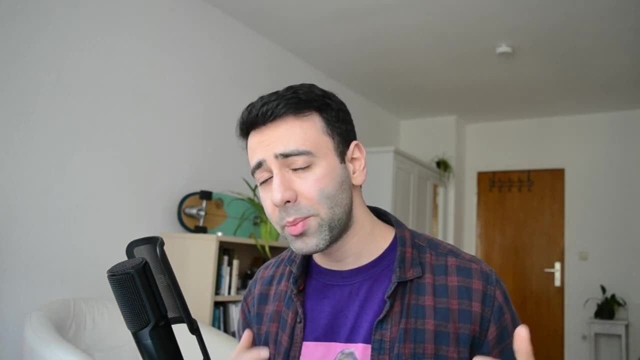 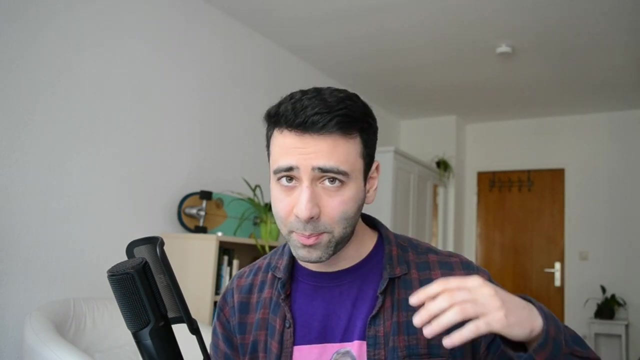 things about REST APIs. Well, the reason they're so widespread is because they're so easy to build, So a developer can build a REST API in a minimum amount of time. The problem about REST APIs is they create this coupling between the backend and a client, So whenever the backend changes, 99% of the time the client also has to change and vice versa. And from my experience, if you have a separate backend team and a frontend team, this kind of creates a toxic rivalry between the teams, because each team has to adjust to other teams' requirements. 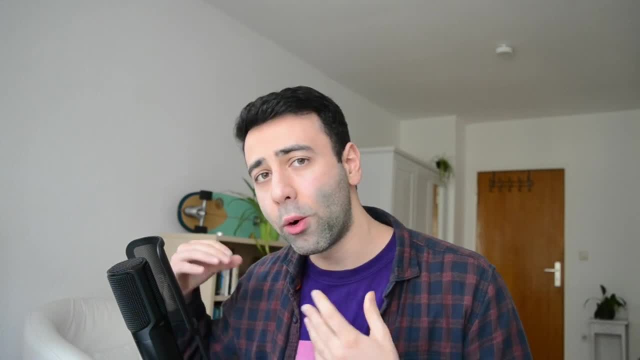 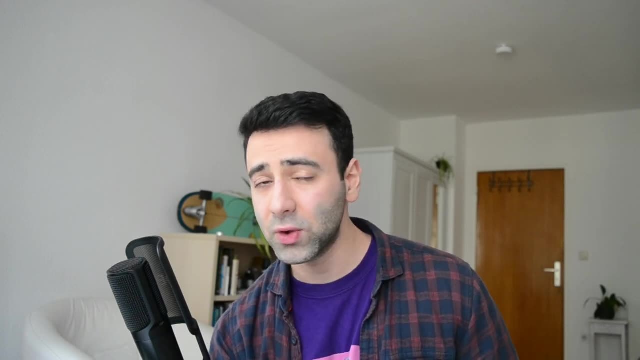 Another important problem with REST APIs is the thing called overfetching and underfetching. For example, when you're fetching the user data, if you want to fetch only the age of the user, but the user object is big, you're going to get all the data of the user. You're going to get the 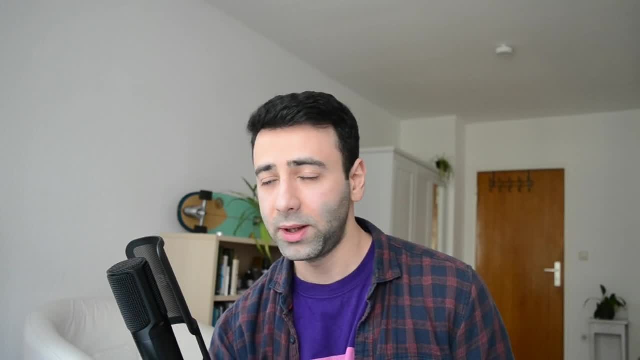 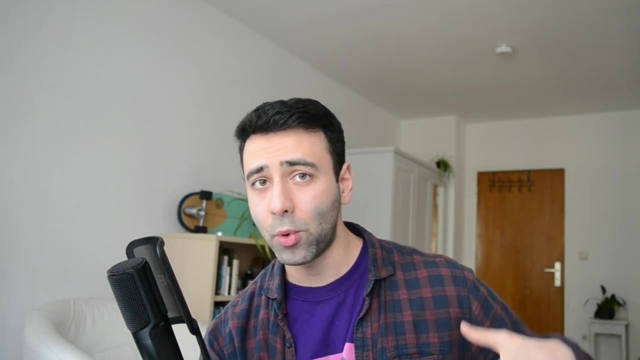 name. you're going to get the surname, you're going to get the profession, but you only want the age. So it's not easy to do that. You would need to create a new endpoint and vice versa, underfetching. If you need more data, you need to go and edit your API to supply you more data. 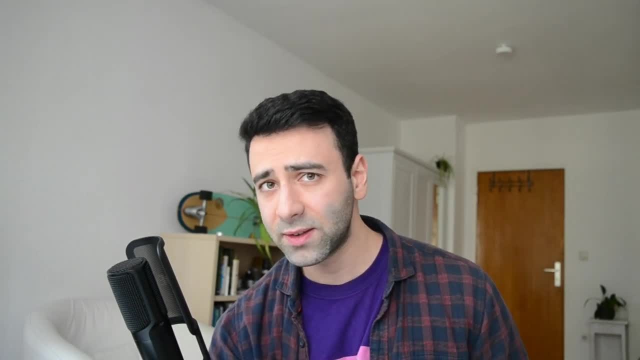 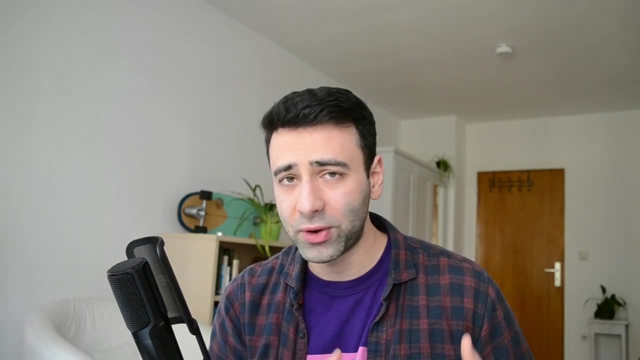 if your client needs more. So you see this. So what can we do here? Obviously, try something else, namely GraphQL. GraphQL is not an architectural feature, It's not a protocol, It's a query language. So QL stands for a query language. 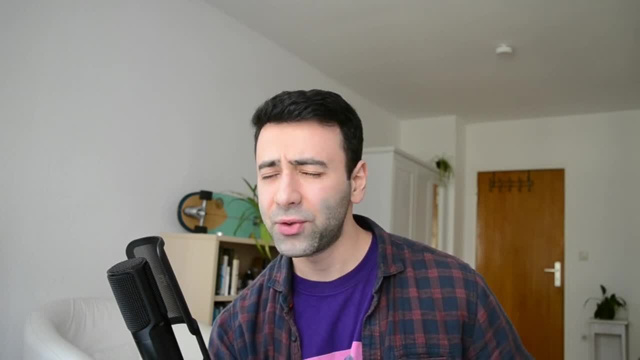 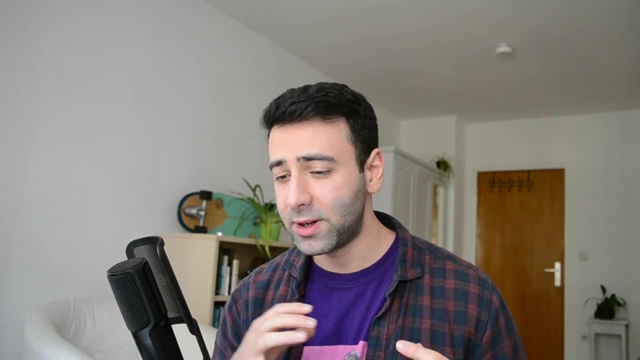 And the cool thing about GraphQL is that it eliminates this underfetching, overfetching issue, So you fetch only the data that you need, which is pretty neat. Also, this creates kind of a contract between your backend and the frontend team, because you have a predefined schema. 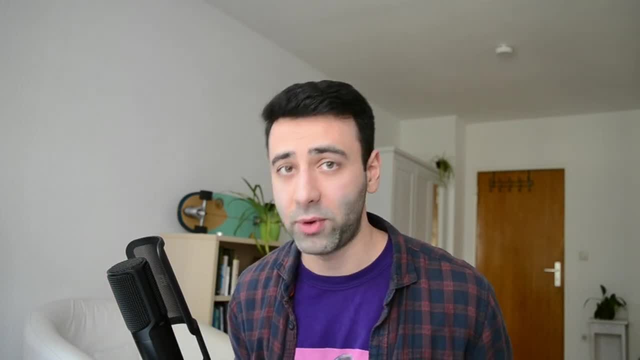 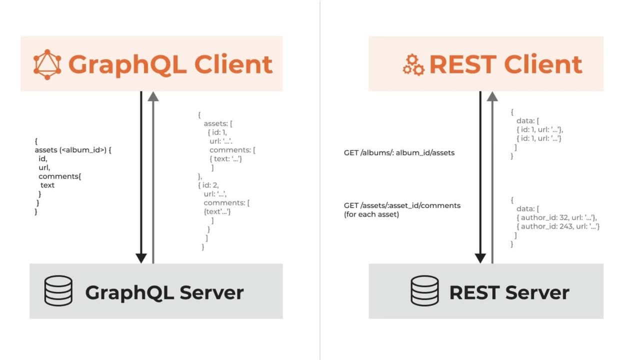 by which you're able to supply your client data from your API. Just by looking at this example, you can see that on the right, when we have a REST client, you have to do multiple requests to fetch first of all the album assets and then you need to supply an asset. 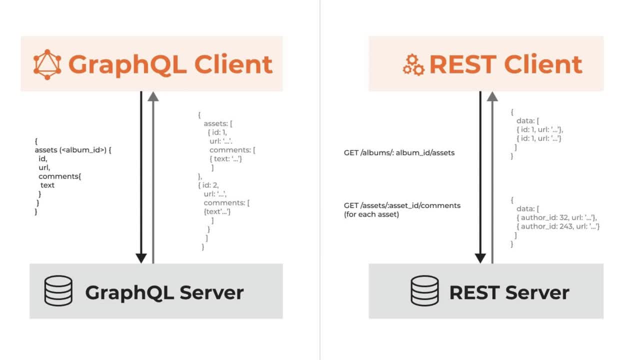 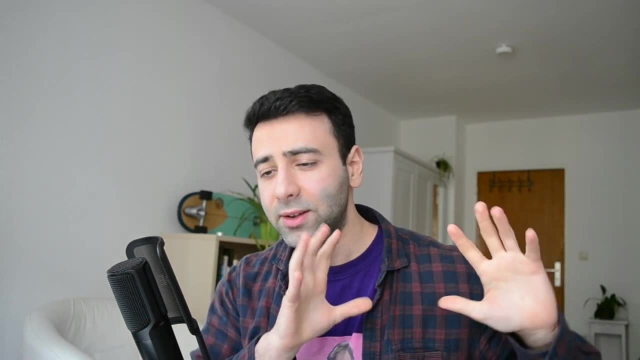 ID, While on the left side we can see that you can do all of these two things in one query, which in fact saves us the bandwidth, So we don't have to replicate our endpoint. And let's say if, for example, you had a website and a mobile app, that they can talk easily to one endpoint, And 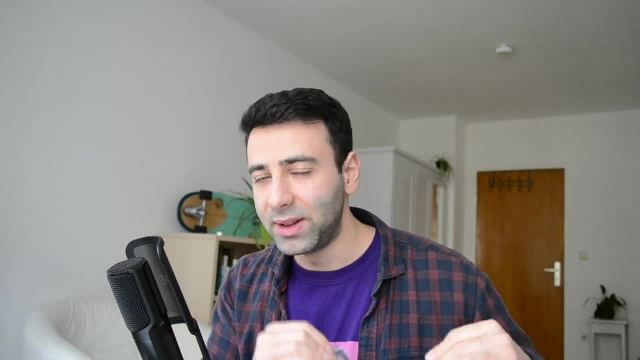 in case of REST API, your mobile app obviously needs less bandwidth because you care about every extra kilobyte that you're filling. So you can do all of these things in one query. So you can do all of these things in one query. So you can do all of these things in one query. So you can. 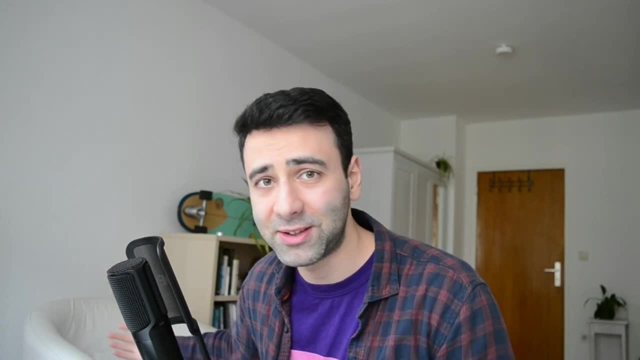 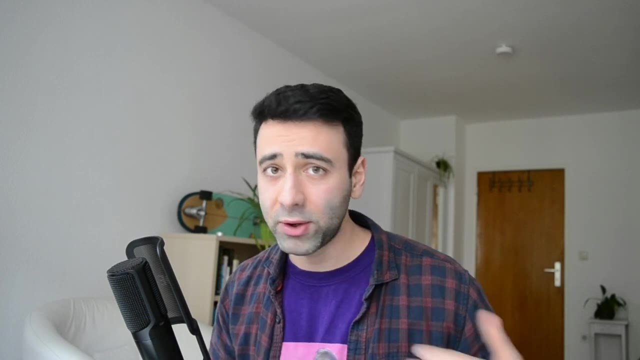 especially if it's some kind of an edge device like refrigerator. you really care about your data that you're fetching versus the website. So it's really hard to implement this in REST And most likely you're going to have to develop new endpoints for your mobile app and your website. 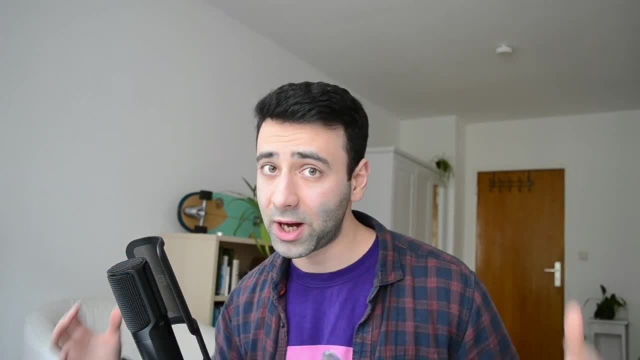 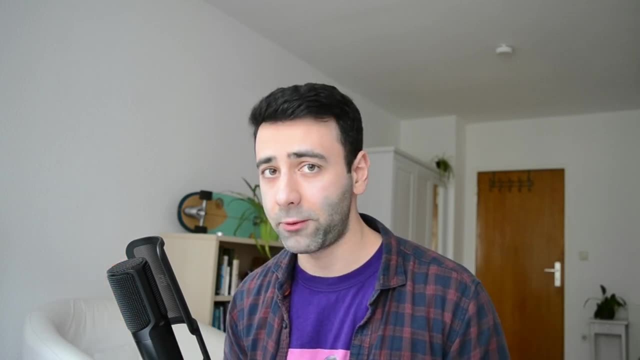 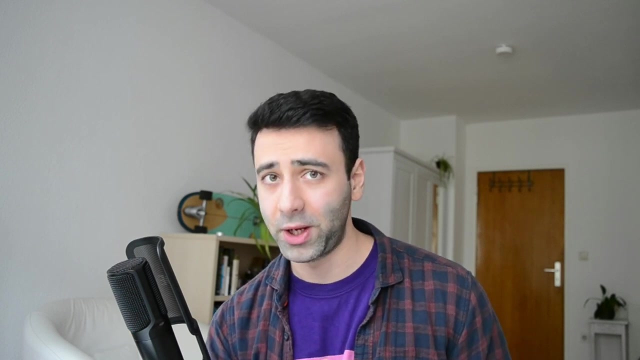 so that they're talking in parallel. But with GraphQL you can overcome this issue easily, because you can easily determine which fields you need from your API. Okay, so what are the downsides of GraphQL? I could identify. one big downside from my own experience is that it's very hard to get GraphQL right If there's one condition that you 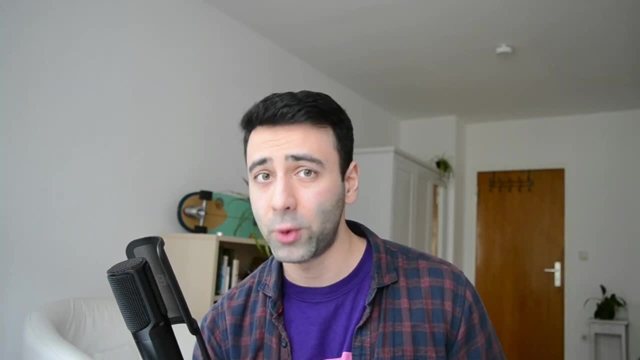 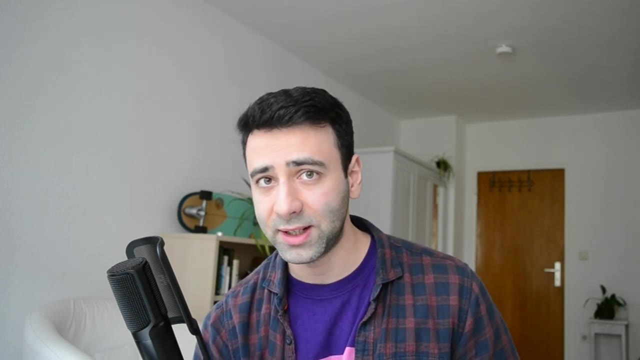 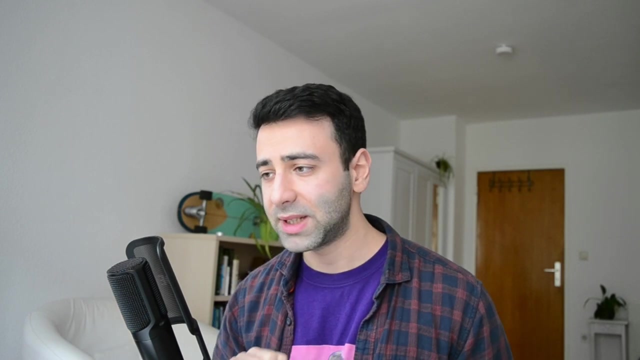 have a really good GraphQL guru in your team who knows a lot about GraphQL- or maybe that's you- then go for it, Because as long as you have a good schema defined on your backend, as long as you have set up everything well on your content, your GraphQL communication will be perfect. But I've 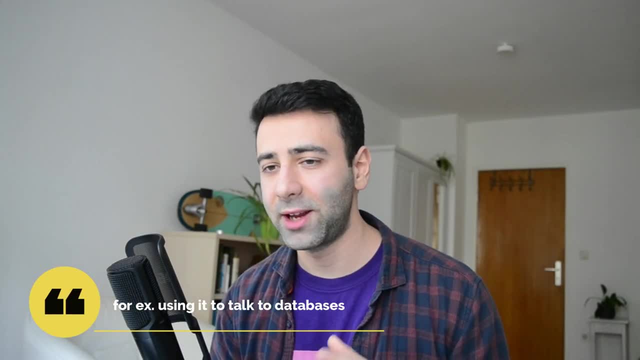 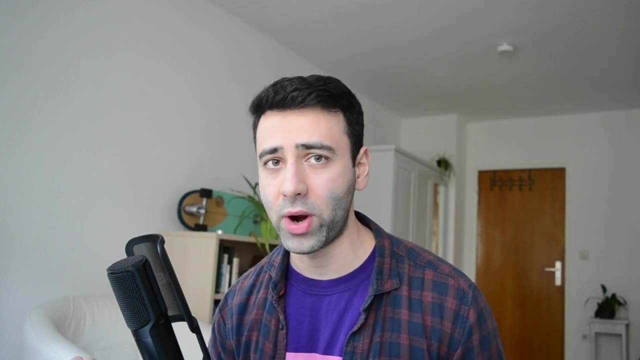 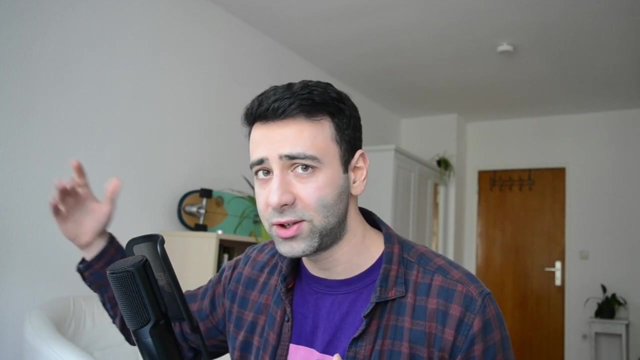 seen teams doing this wrong, And another downside of GraphQL that I personally ran into is the fact that it's very hard to get them right. They have their own built-in caching system with write query and so on, So just to make an ordinary HTTP request, you have to write a lot of boilerplate. code And since it has its own built-in caching system, which doesn't play that well with your browser's native caching system, you usually run into weird bugs. So bottom line: when should you choose REST APIs versus GraphQL If you have a very complex data representation? 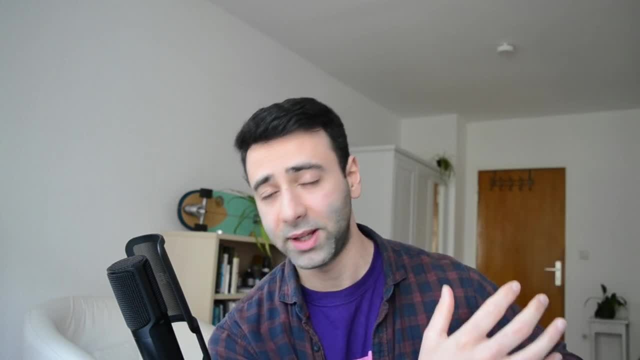 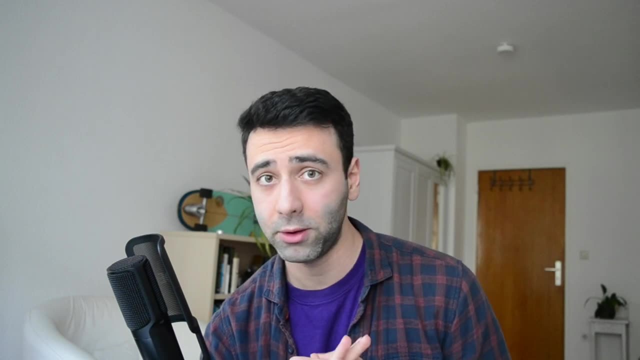 let's say you have users, then your users can have playlists, playlists can have assets. So a very big nested object data objects that you're sending around- go with GraphQL. It's not easy to do that with REST and you're going to end up with a lot of overhead If you care about bandwidth. 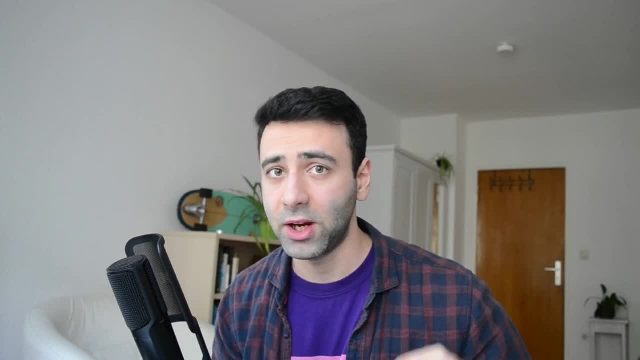 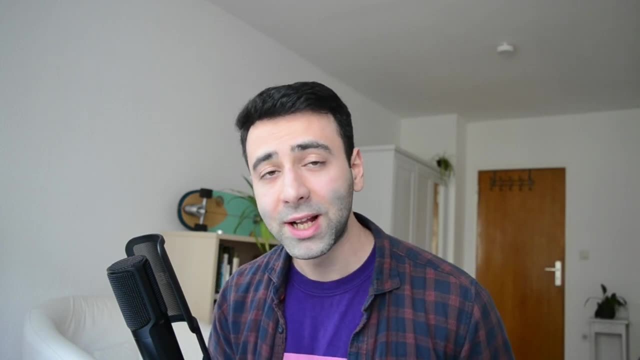 so if you have mobile users or if you have some edge devices that care about every kilobyte transferred over the network, go with GraphQL, because you can select specific data that you want to fetch. If you're a startup that needs to iterate very quickly and you 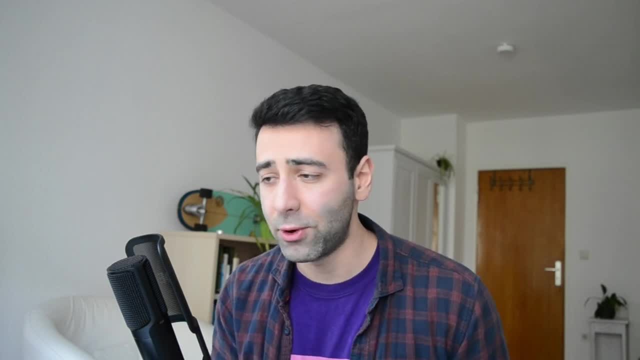 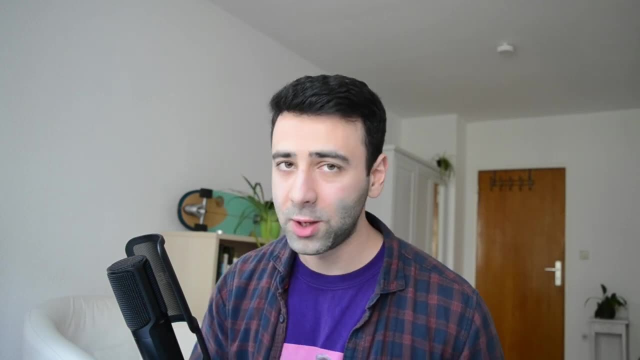 need to be able to find developers very easily and you don't have much time. go with REST. Okay now, what is tRPC then? Well, RPC stands for remote procedure call, while t simply adds TypeScript. Now, before we continue, a quick word from our sponsor Namecheap. I thought I've 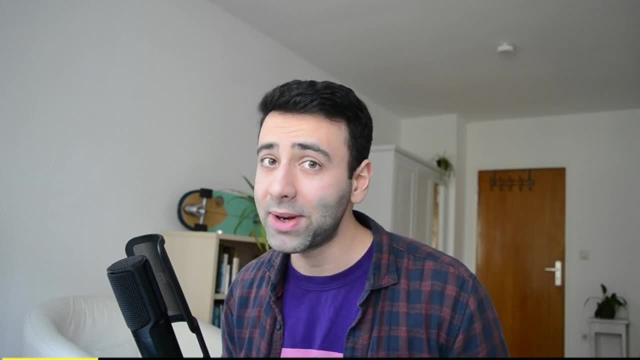 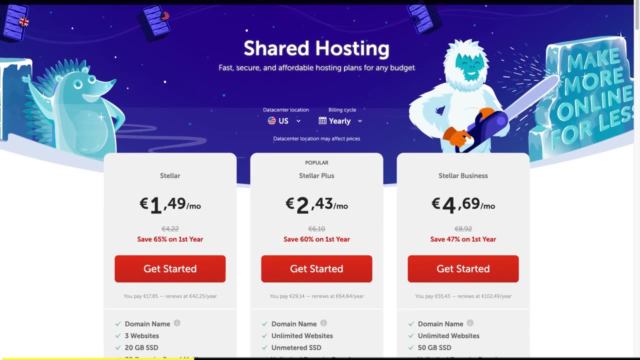 already told you about this, but apparently I haven't, So I'm going to have to tell it again. I'm sorry. You can host your website for under two bucks a month. Yes, and this is real. So on top of that hosting, you're also going to get an SSL certificate, which means your connection with 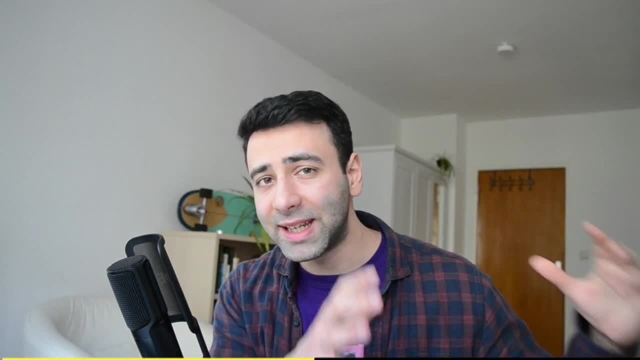 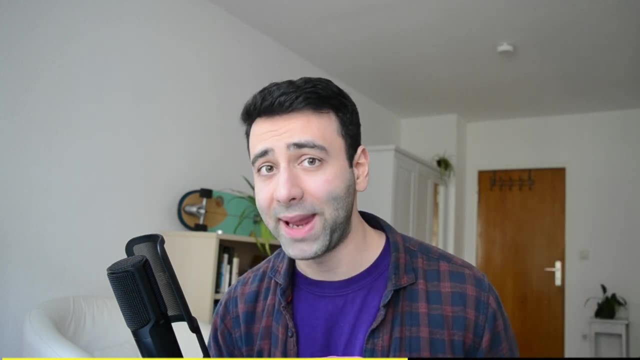 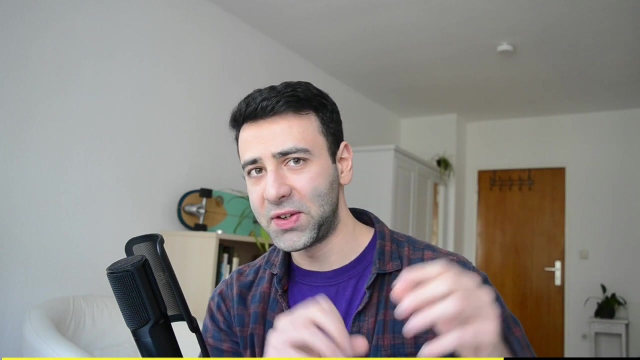 the server is going to be encrypted. You're going to get a 20 gigabytes of space on your disk. You're going to get a 24 hour customer service and a free domain. How cool is that? If you also agree that it's cool, then do we have a deal? Well, if you're still not convinced, here's the thing You can get. 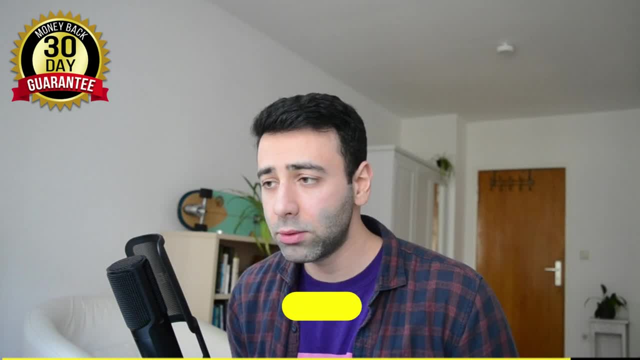 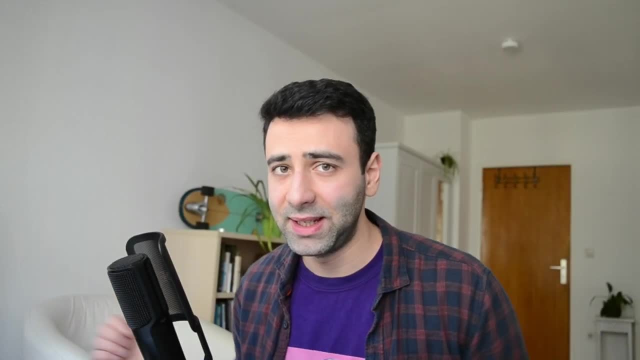 a 30 day money back guarantee, So if you don't like it, you can get your money back. Now I guess we have a deal right. And now back to the video. The main idea behind tRPC is that it brings 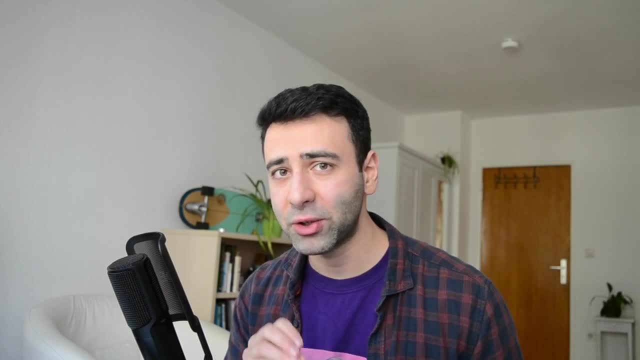 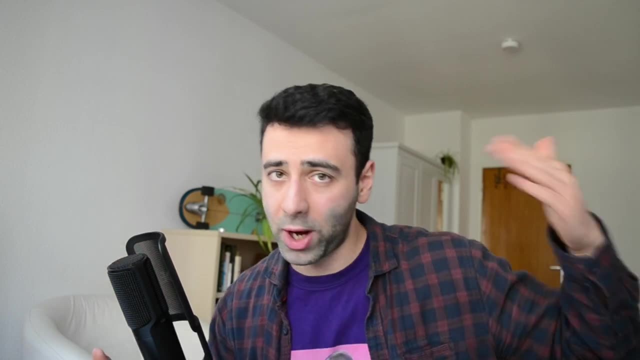 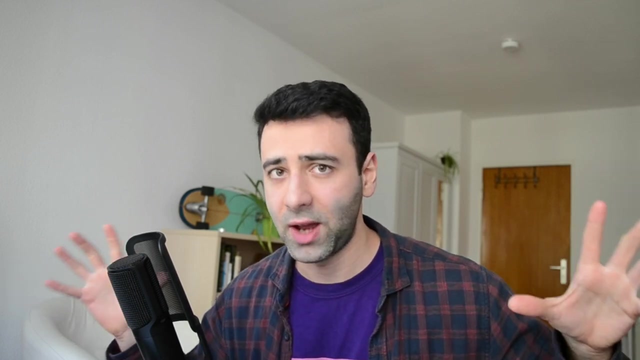 backend and the frontend much, much closer to each other, especially if you're using JavaScript in your server and the client, namely TypeScript. So behind the scenes, imagine- your server has routes and controllers are responsible for handling routes. right in your normal ExpressJS app, This 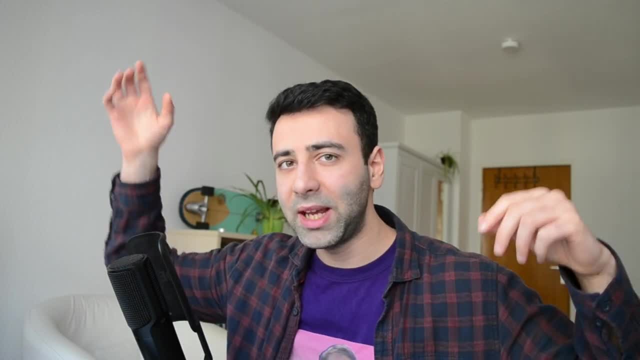 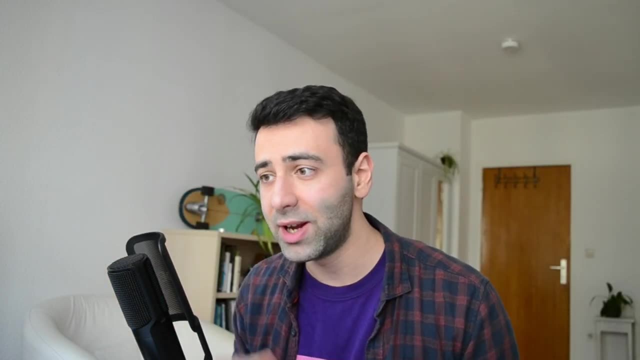 is how it works. So in tRPC, your client is going to be able to call exactly these controllers as if it was a server. So if you're using javascript, you're going to use your server and your client is one application, so they're really coupled to each other, and on top of that you have a typescript. 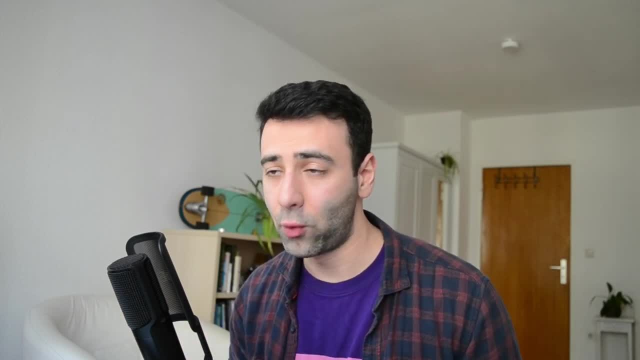 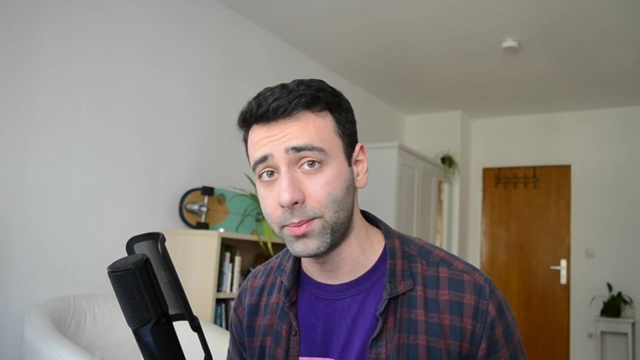 which adds a schema. so there's really no way of supplying wrong data from your client to the backend, because there's typescript that defines an exactly typed schema for both of them, and usually when you're using trpc, it's very common to use a monorepo if you already have a monorepo. you're lucky. and if you're using typescript, and on both of your ends, you're lucky. otherwise, try to use a monorepo for trpc, because your client is going to be able to import exactly the same schema that your backend has defined and simply call it so. otherwise, if you have a rest, you can. 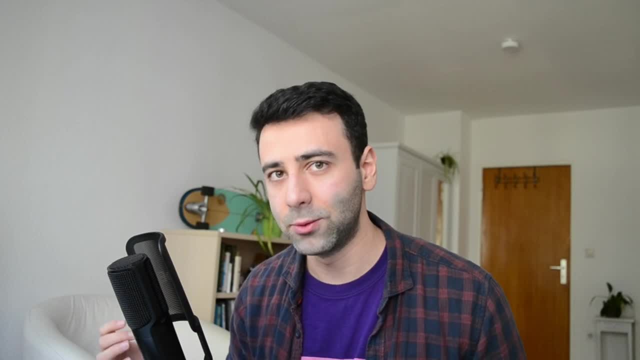 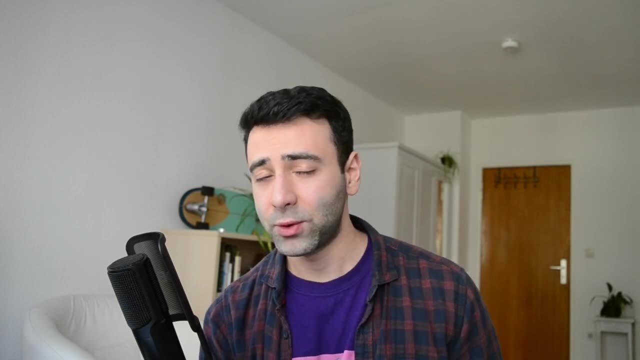 slowly migrate it. but if you don't, then it's up to you whether you want to rewrite your application to trpc. so what are the advantages of trpc, apart from the fact that it's strongly typed? so trpc runs on top of http2 and it has a lot of out-of-the-box optimizations and capabilities. 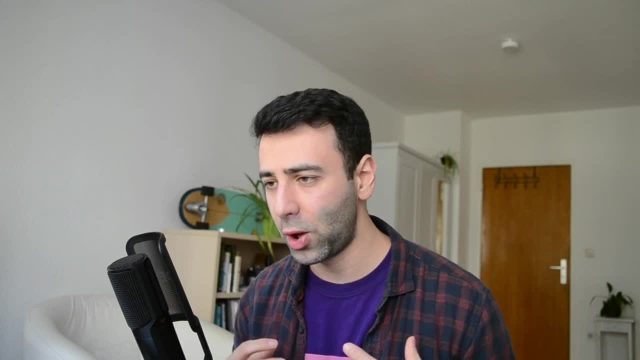 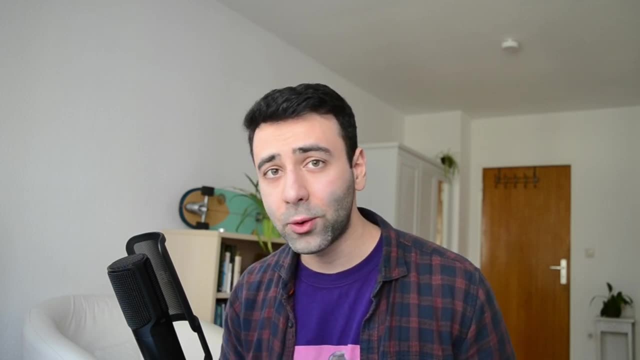 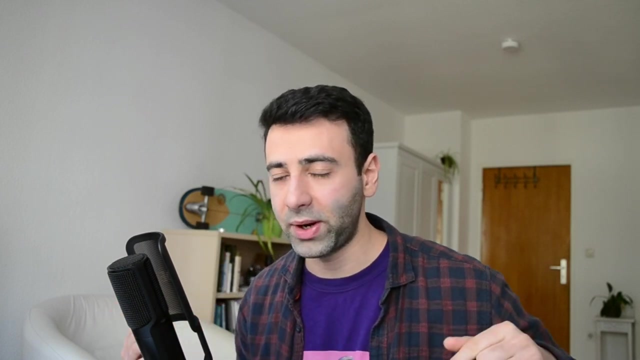 that's going to make your code unique and very close to each other, so this is definitely a nice thing and it's very lightweight compared to graphql. of course, another cool thing is that your ide is automatically going to be able to redirect you from your frontend code to your backend if you press ctrl, right, left, click on one. 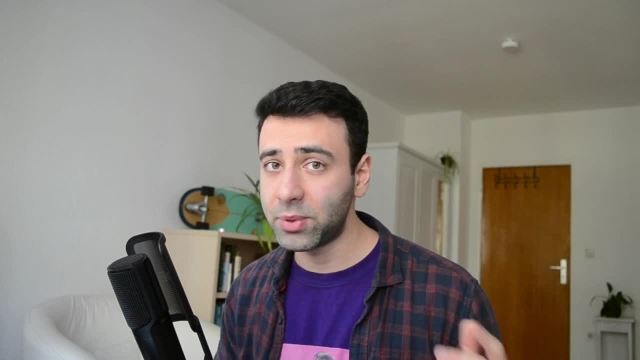 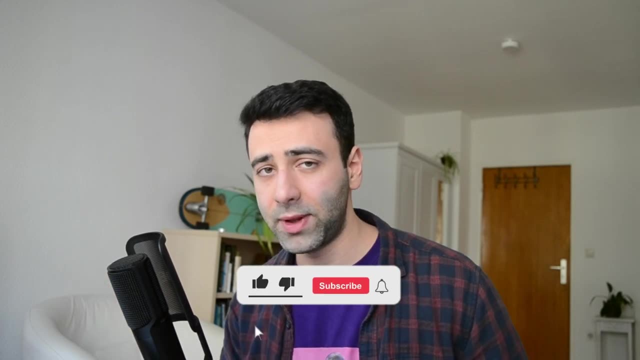 of your functions that you're calling from your frontend. i'm going to make a separate video going into details of trpc and looking into code and how it can work with react in another separate video that's going to you come out in a week, so make sure you subscribe if you're interested. also, trpc has a much lower 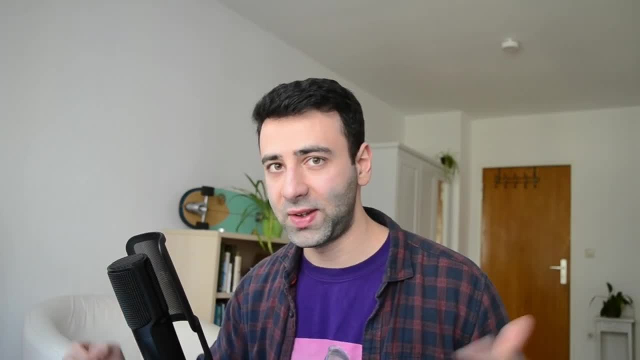 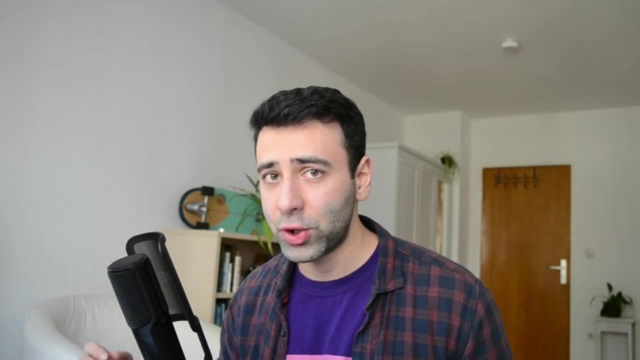 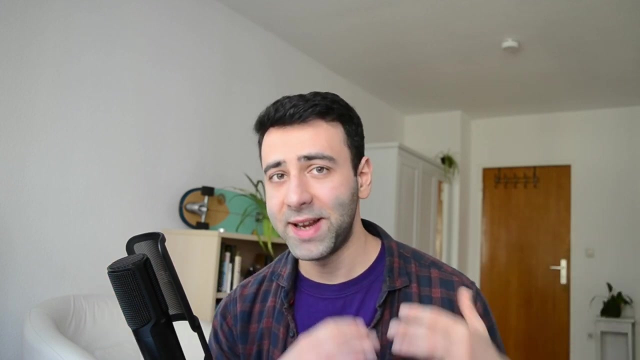 bundle size and it doesn't suffer from this bulky packages that graphql forces you to install on the client and your server. so when should you use graphql versus trpc? trpc unfortunately does not fix the problem when you need to request only specific data from your api. so if you have nested, 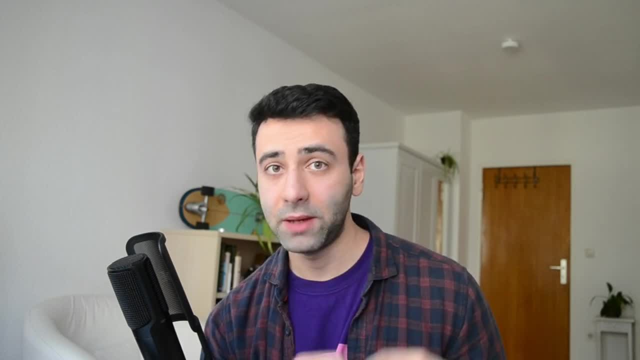 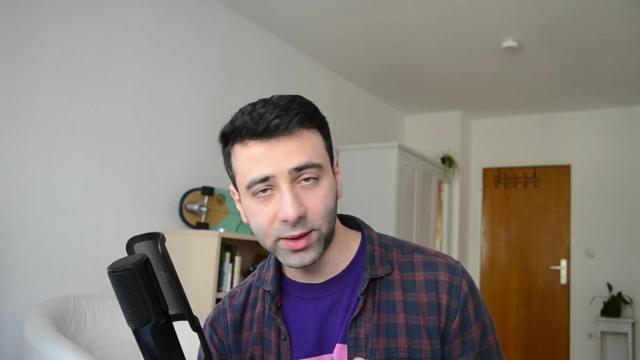 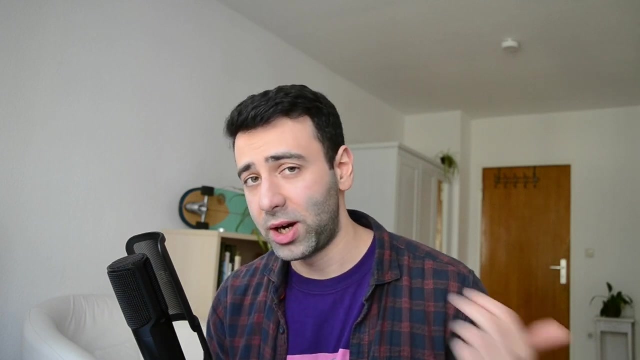 data and complex data, you have to go with graphql. if you're caring about your bandwidth, you have to go with graphql. and when should you choose rest versus trpc? well, if you're already using javascript on both of your ends, and especially typescript, you can go with trpc. and last but not least, g rpc. here we replaced. 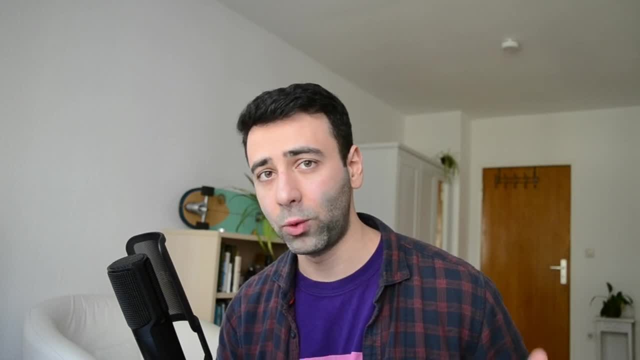 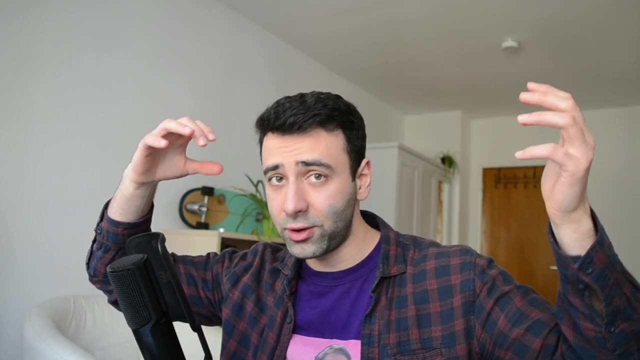 t with g, and g here stands for google, so google remote procedure. again, it has the same concept as trpc, which means they're gluing your client to your server and your client is able to invoke specific functions of the server, as it was one application and also 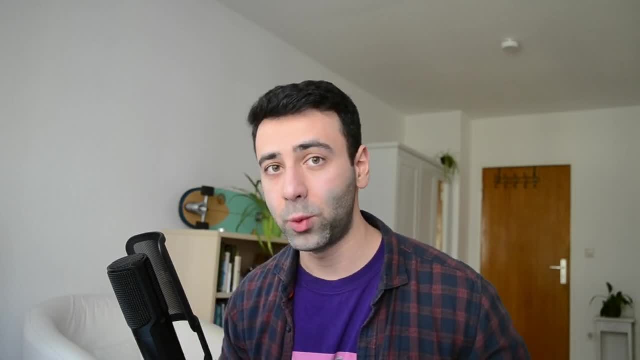 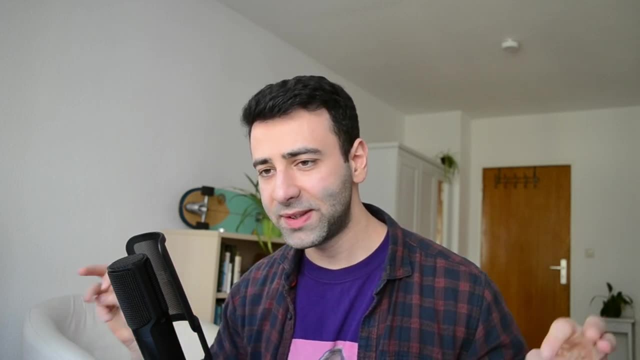 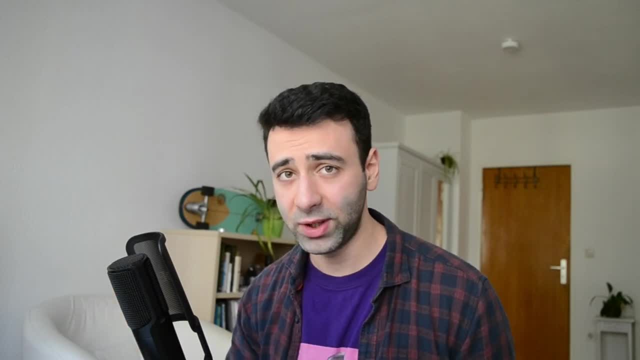 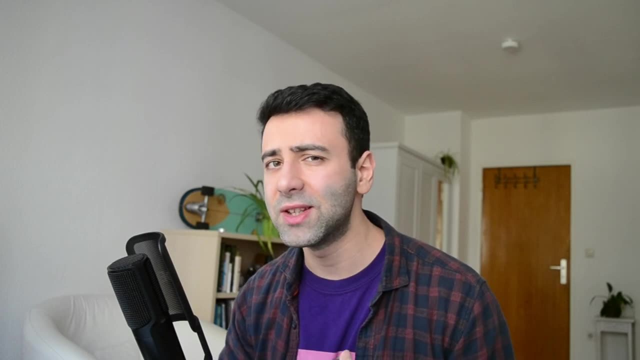 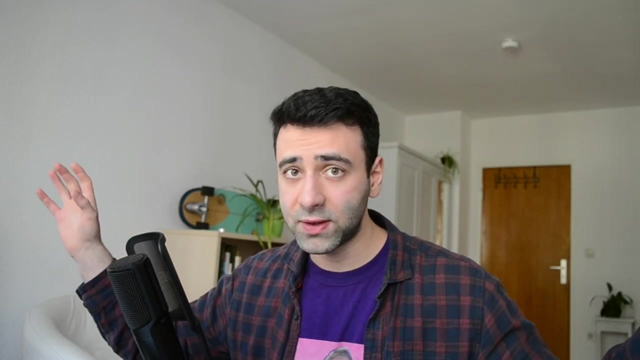 http2 capabilities, because g rpc really works much faster than anything else. but modern browsers- even the modern browsers- are still not able to do that. so you need to install a g rpc web package to be able to do that. but if you need g rpc simply for your microservice, 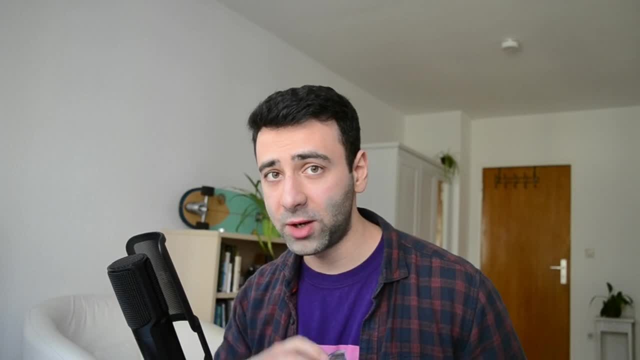 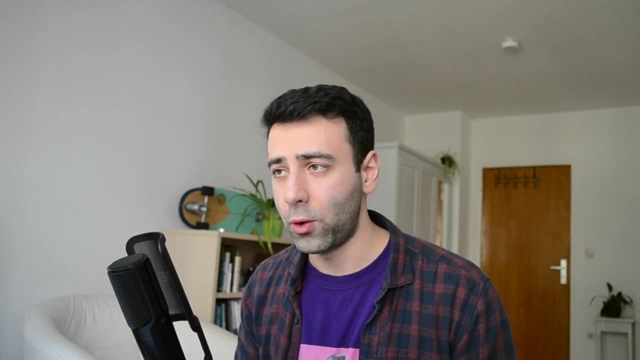 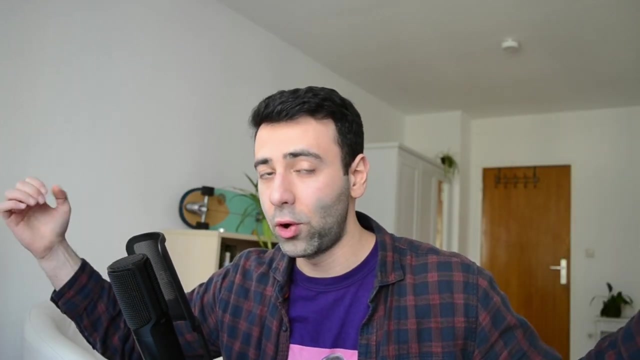 to talk to each other. g rpc is the right way. also, you can use g rpc over trpc if your microservices are written in different languages, for example in java and go and node. so you're not only limited to tab script and you can still use the same functionality that remote procedure calls give.